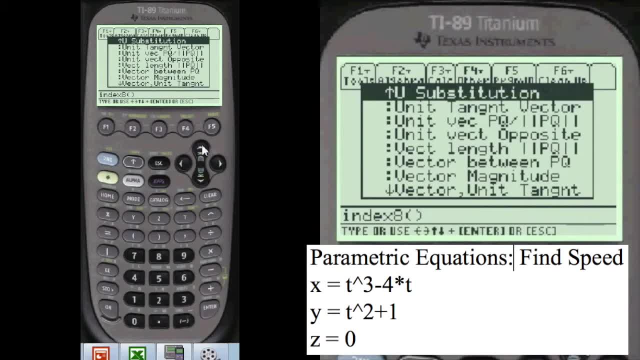 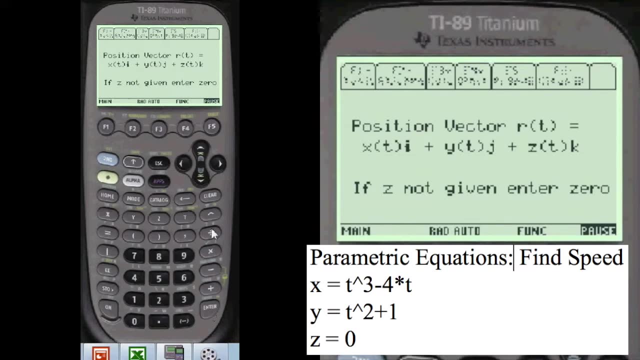 add time to it, which I'll show you in my program- here There's speed- And write all this on your paper and your R-T formulas. you know X-T-I, J and K, it's X, Y and Z, And we add our functions for X and Y. We have to press alpha. 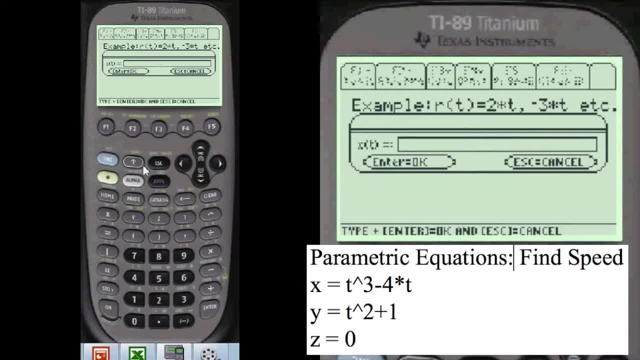 before we add anything on these entry lines here: Alpha Problem is T cubed minus 4 times T And alpha T squared plus 1. Looks like the T is missing. I'm going to go back into here and put the T in. There we go. 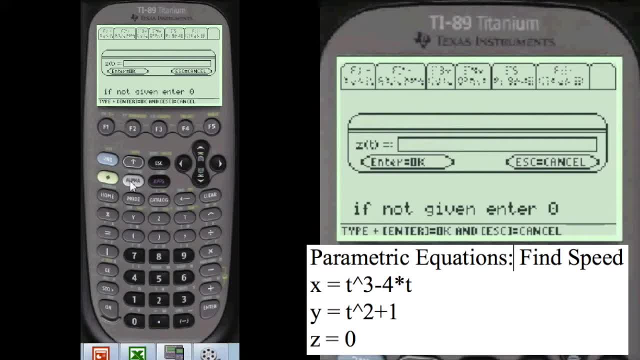 And alpha 0 for the Z component And alpha 0 for the Z component And alpha 0 for the Z component. We're almost done with the C component or A component if it's not given. These are all set up problems. They don't happen in real life. a bunch of nonsense for. 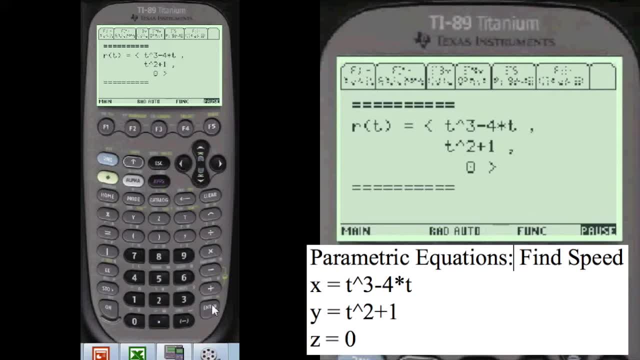 calculus. A lot of that is like that in calculus. So I always show you what you've entered. You can change it if you want. he say it's OK And we're going to scroll down here to the calculation. now you have different patterns. 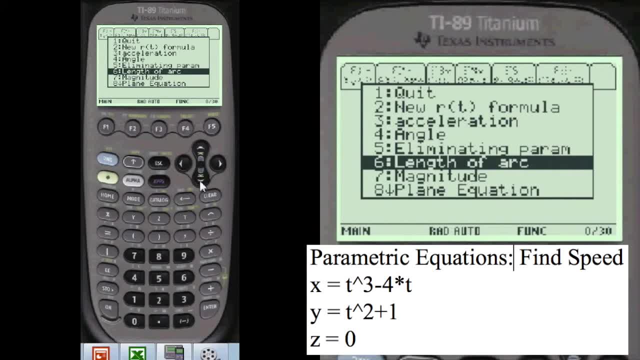 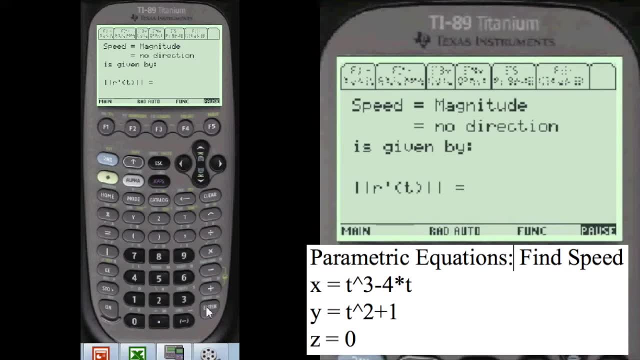 The things in the menu that you can do with this entry of t variables: Speed, there it is there, And, of course, given by the derivative of the magnitude of it, which is actually this square of the derivatives. Calculate this, the Sudoku of math: x, prime. here's the derivatives of that, And the magnitude is then the derivative squared.